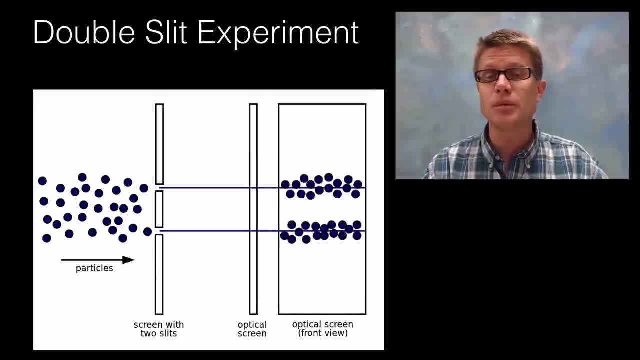 to look like on that screen if I turn it so you can see it. Well, you can see, it is going to move. Well, you probably guessed this. In other words, the particles are not all moving in a straight line, But they are moving through the slit, They are hitting this screen And 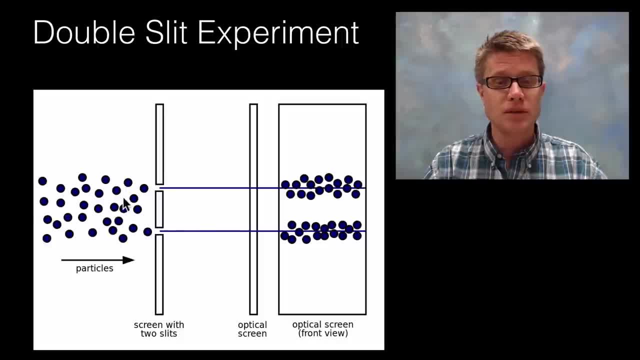 then we are seeing that if we turn it sideways. And so what do you think happens if we were to close up one of these? Well, the particles are not going to make their way through. If we close this one, what is going to happen? The particles are not going to make it through. 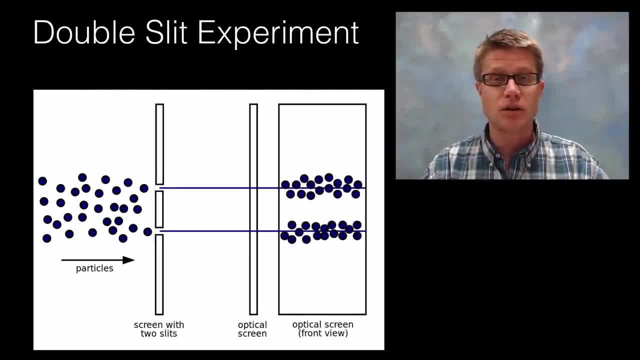 there as well, And so if we remove both, then we are back to where we started, So you should not have learned anything new. This is how the world works. Now. let's say, we are using waves now, And so imagine that we are shooting a ball, And we are shooting a ball, And we. 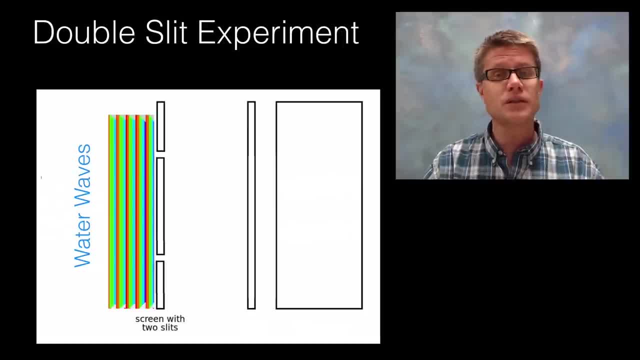 are shooting instead of shooting spray paint through these slits. We have now got a wave tank where we are generating waves on the left side. Those waves are moving through the two slits And then we have detectors on this screen that are showing us what is. 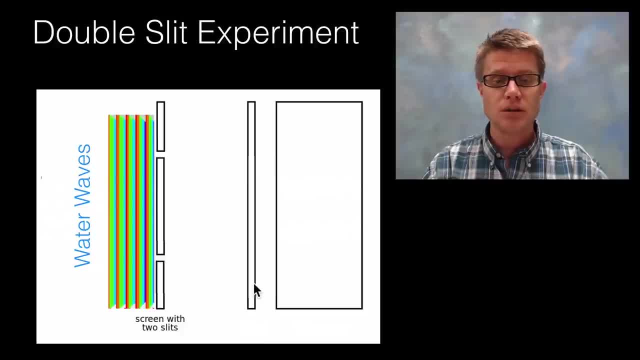 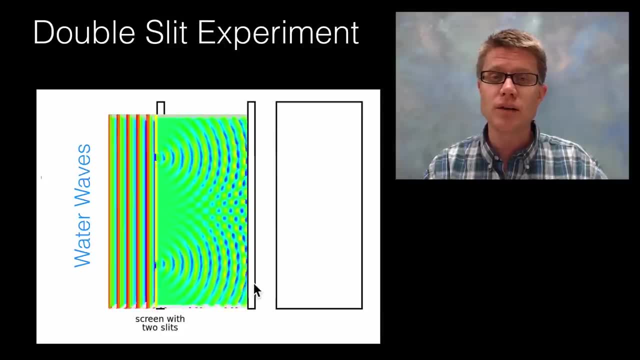 the amplitude of those waves, How much energy is being transferred through. So if we kind of simulate that it is going to look like this And so what we are seeing is interference, You can see that as those waves move through, we are increasing the waves in some places. 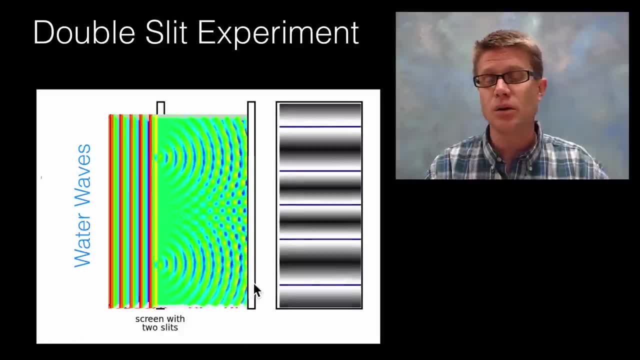 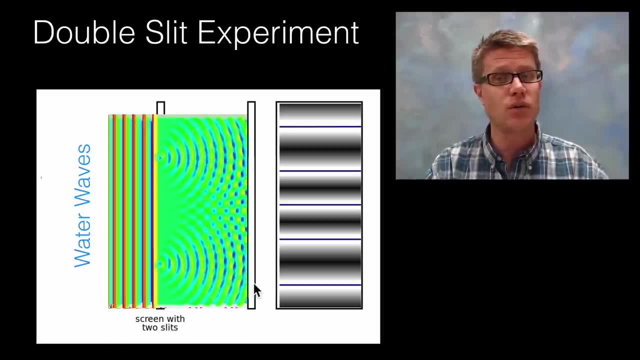 decreasing the waves in some places, And what you see is an interference pattern that we would look like this: Because those are moving as waves, they can interfere with each other and so you don't have two discrete units. That's how waves look in a double slit experiment. 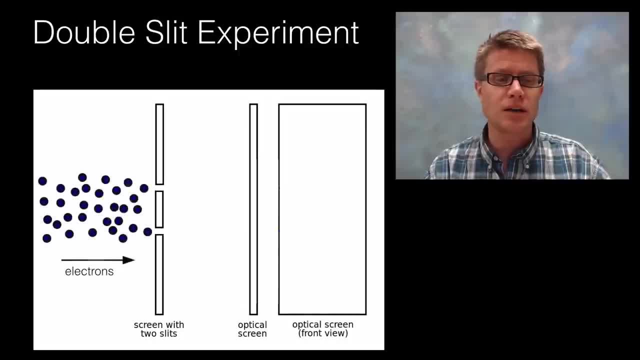 And so then scientists said: well, let's look at something very, very small. Let's look at an electron, which we tend to think of as being a particle, And so let's shoot particles through this double slit experiment and see what we see on the other side. So you might. 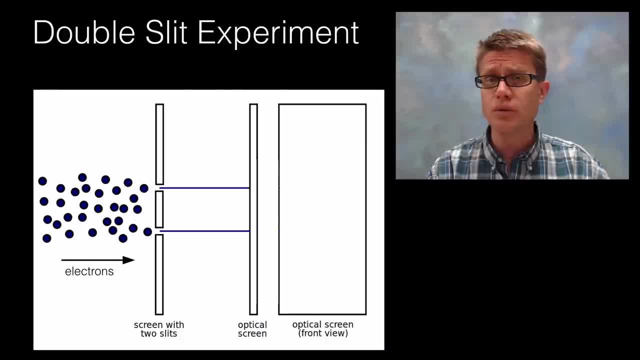 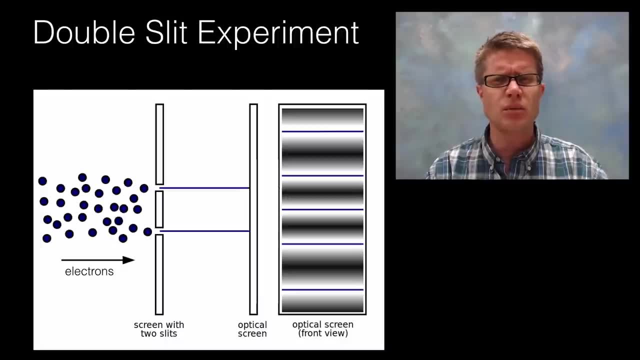 imagine they're going to move through. If we turn it towards you, you might think it would look just like those marbles or that spray paint did, But what you see is an interference pattern. So we see these things that we think of as particles and they're starting to act. 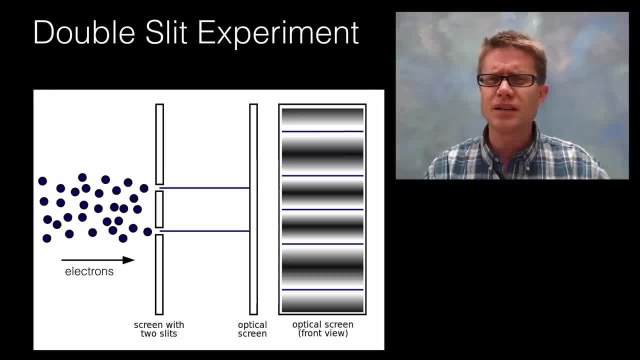 as waves, They're interfering with one another. And so scientists thought: well, maybe they're all going every which way and so they're interfering with each other. What if we just shoot them one at a time? So let's just shoot a few electrons at a time, And what they find is that, as they 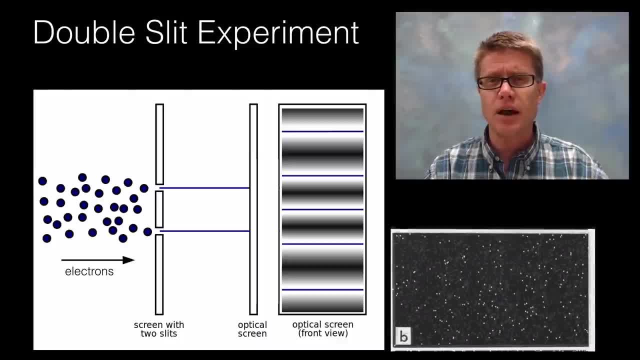 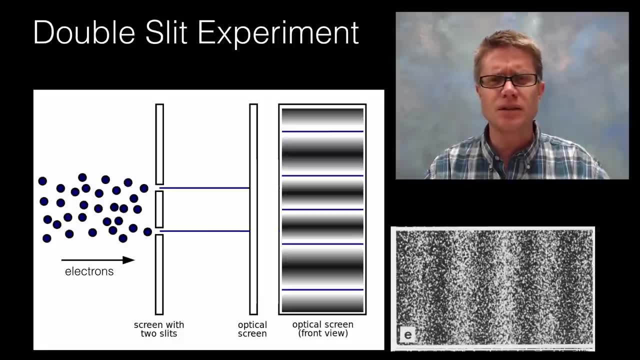 do that over minutes and minutes, and then hours, and then hours. what's happening is this interference, This interference pattern starts to emerge, And so this is crazy to scientists. So what's going on? Are they somehow interfering with other electrons in the future or in the past? 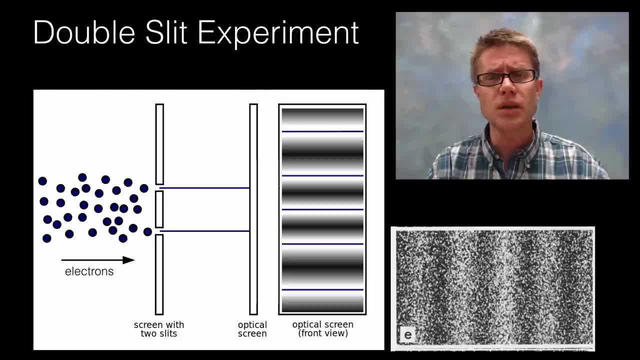 Are they somehow dividing in half and then interfering with each other, those two parts of that electron? And so scientists want to test that. So what they do is they observe it. In other words, they put flashes of light that are going to be released when they incident. 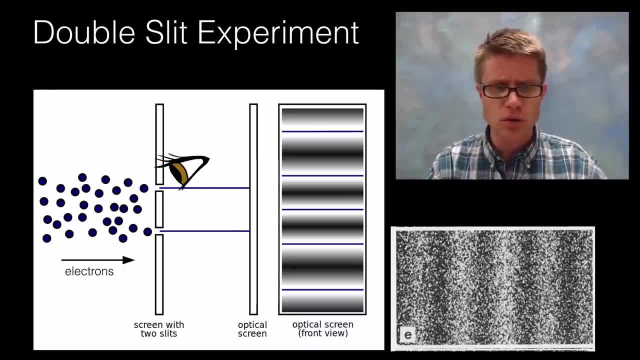 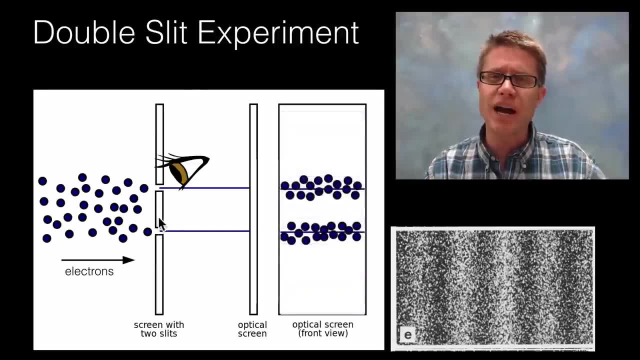 with an electron and they see what happens then, To see you know which one of these holes is the electron going through. And as they start to observe it, something even weirder happens: It goes back to acting like a particle again. And so, again, what is this showing us? That these particles that we think of, 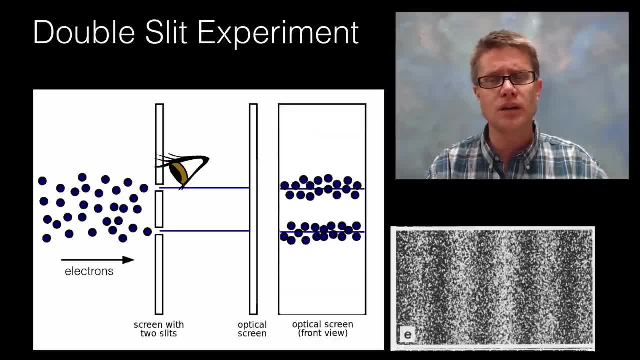 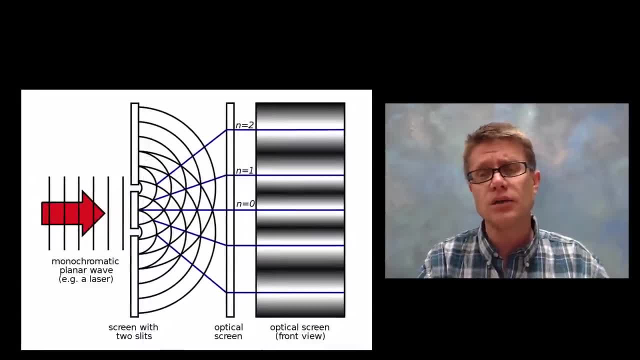 as discrete little units are actually behaving like waves, And it opens up this world of quantum mechanics, And so you could do this if you wanted to. This works with any kind of a light source, like a laser light source, where it's moving in one coherent plane And 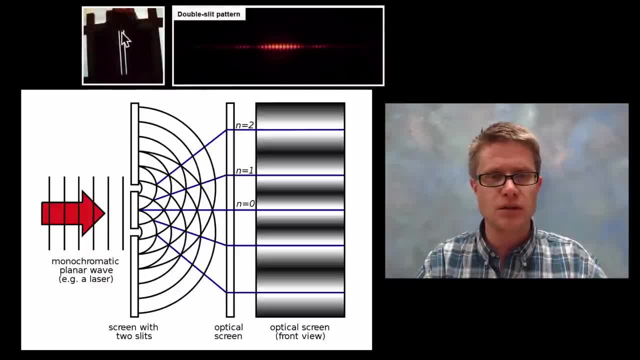 so what you could do is just shine a laser through these two slits. You could do this in a physics classroom, And what you'll get is this diffraction pattern. on the other side, It's something that we can observe, but it's being created at the quantum level, And what? 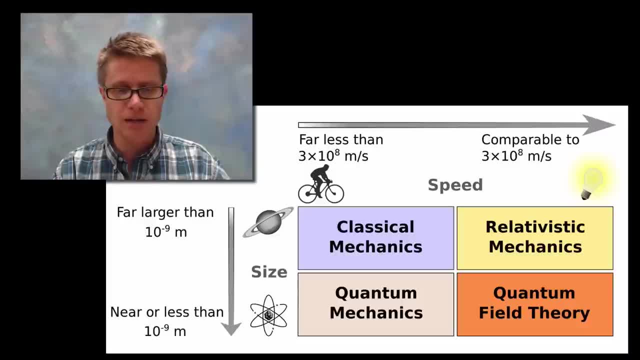 do I mean by that? Well, we live in the world of classical mechanics. We live in a world where everything travels much less than the speed of light And things are much larger than the size of an atom, And so we live in this world of classical mechanics, Mostly. 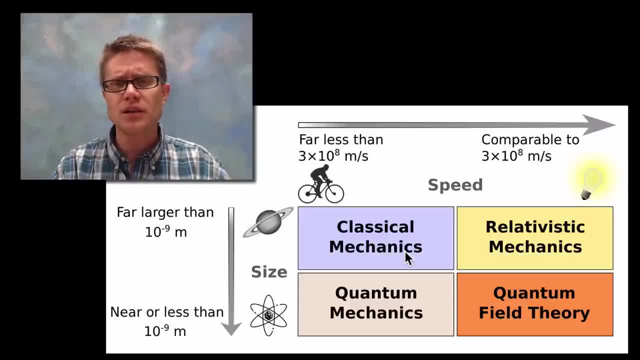 you're going to learn in physics one and two, But know this: That as things get really really fast, we have to adjust and use relativistic mechanics, And as things get really really small, we have to use quantum mechanics. And so the double slit experiment doesn't work. 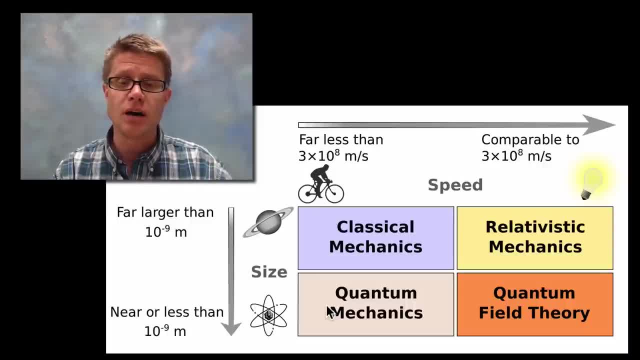 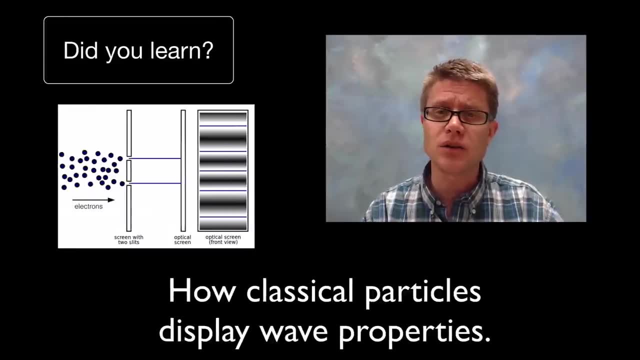 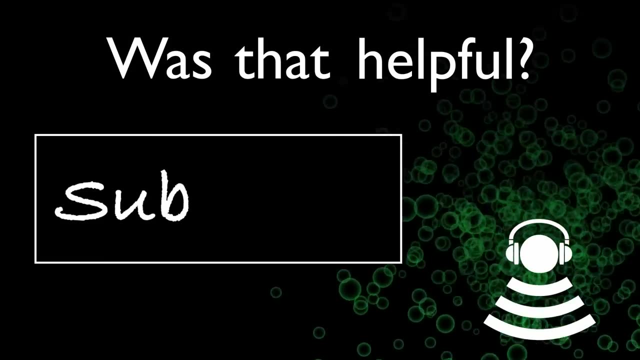 in our classical mechanics world, But it does work in the world of the very, very small, And so did you learn this, How classical particles like electrons and photons can have wave like properties? I hope so, And I hope that was helpful. Thank you.